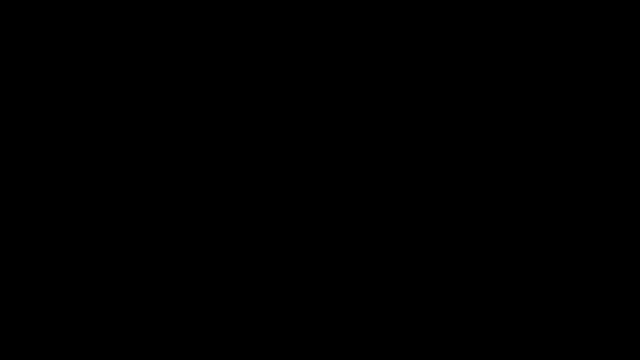 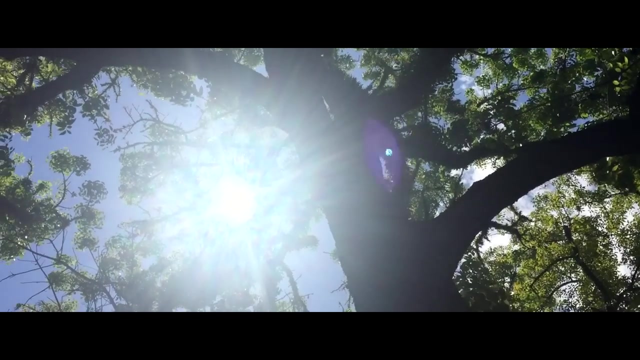 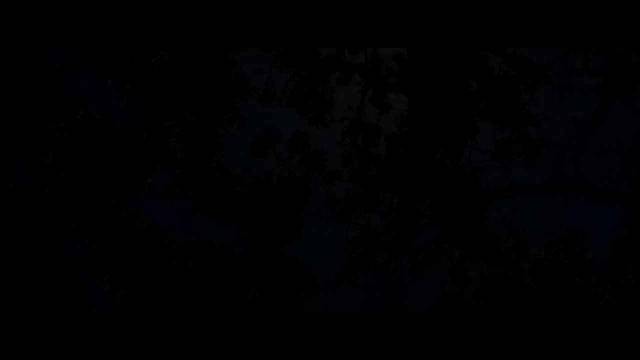 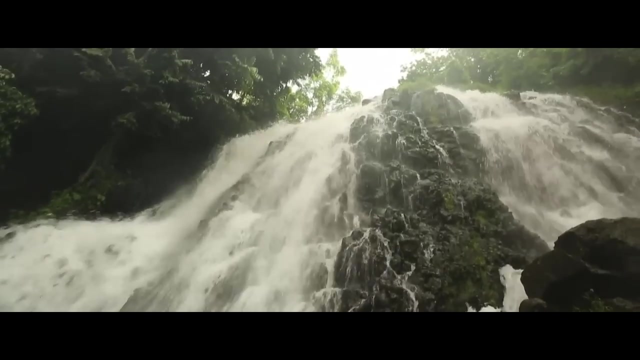 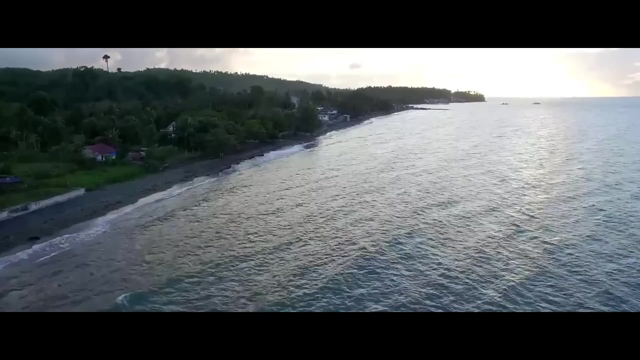 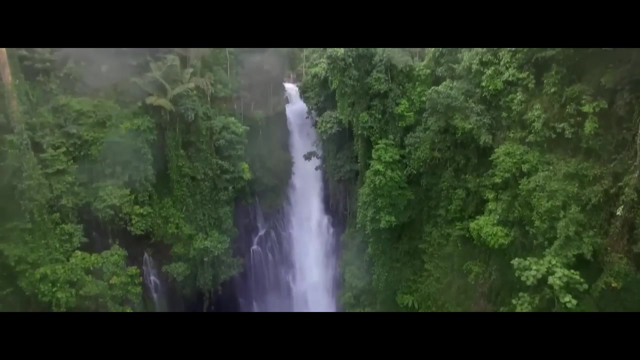 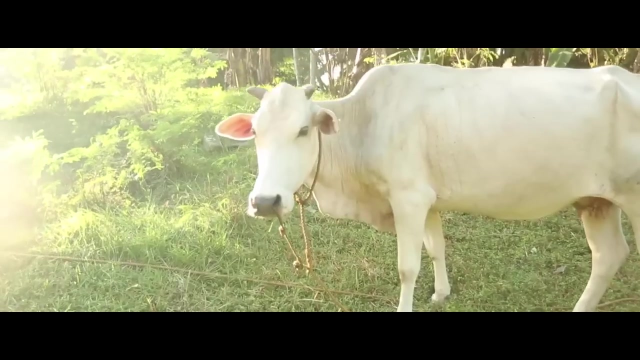 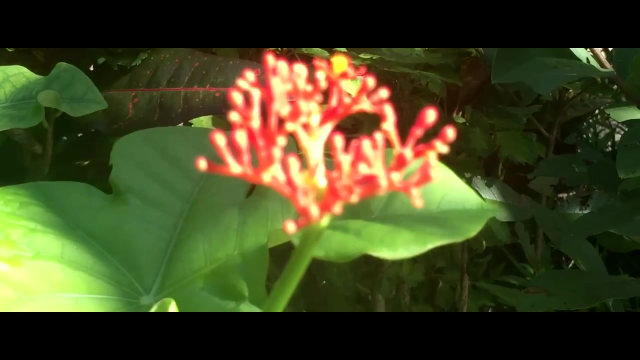 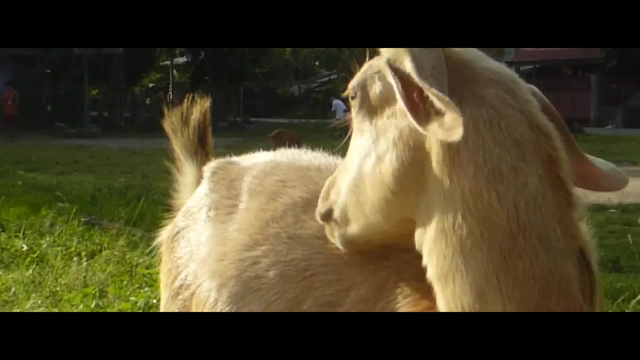 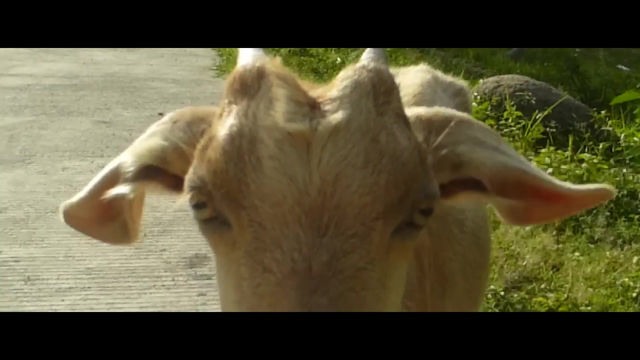 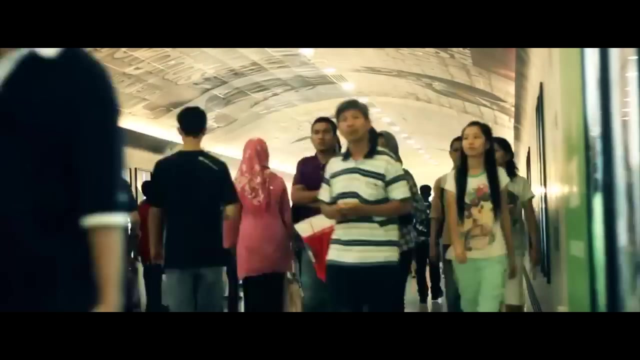 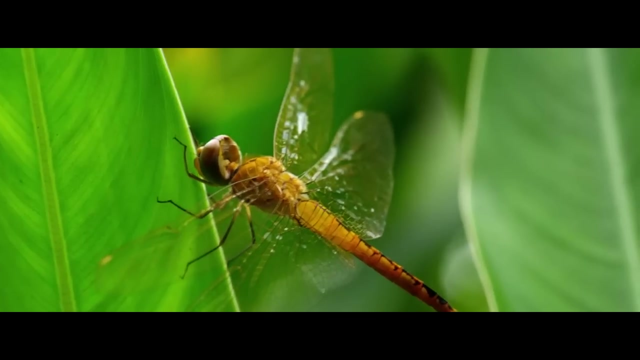 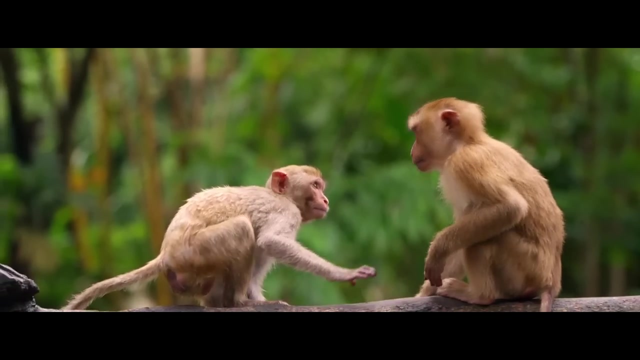 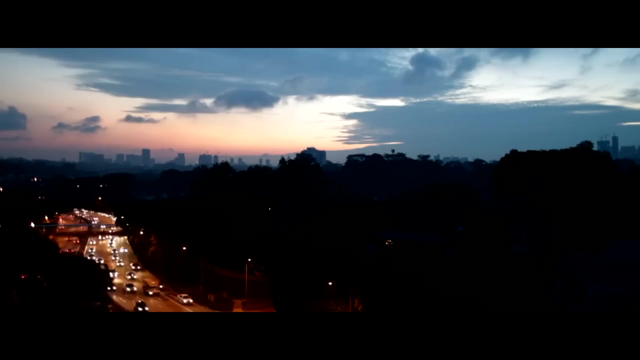 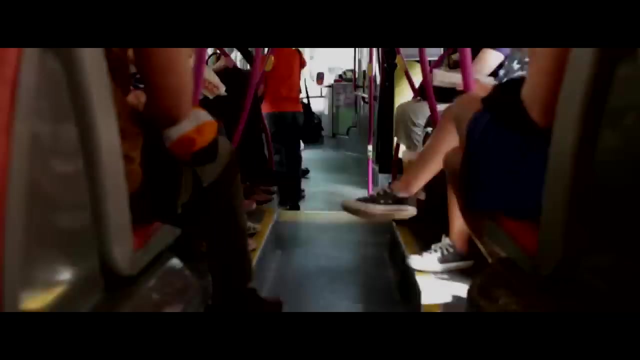 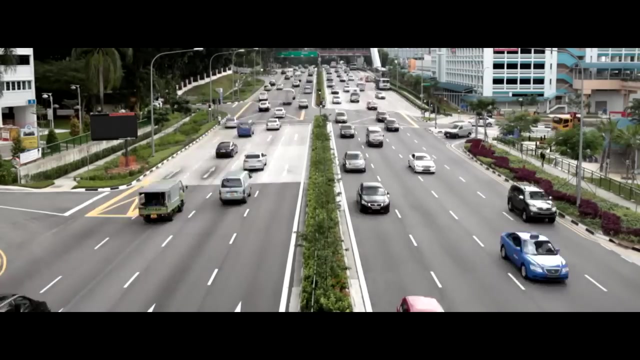 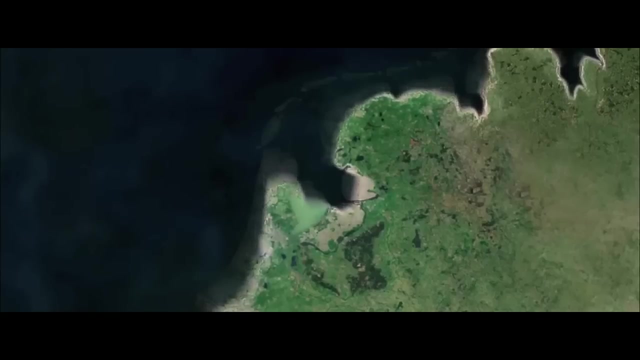 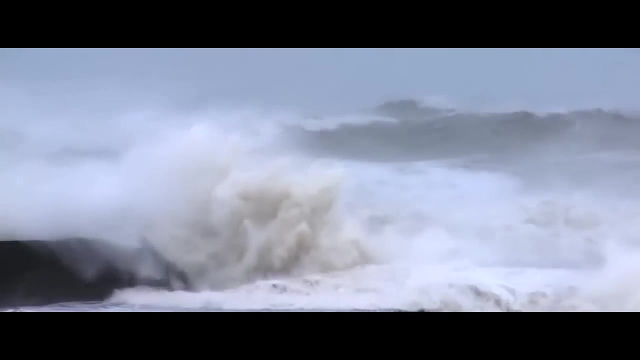 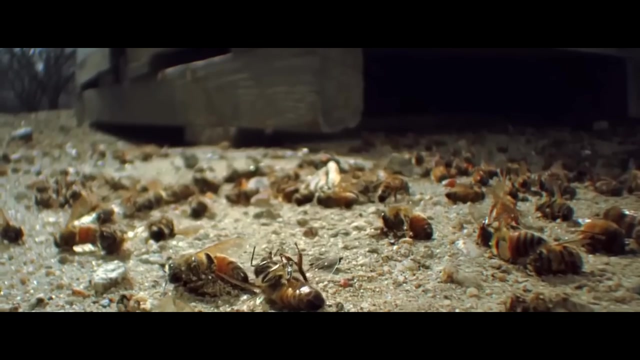 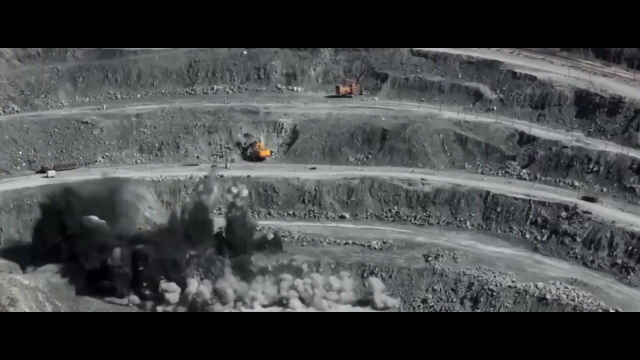 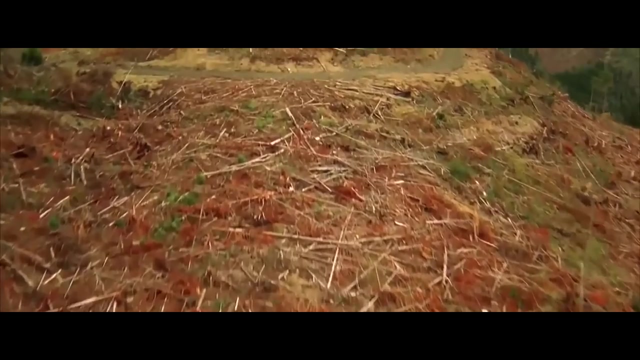 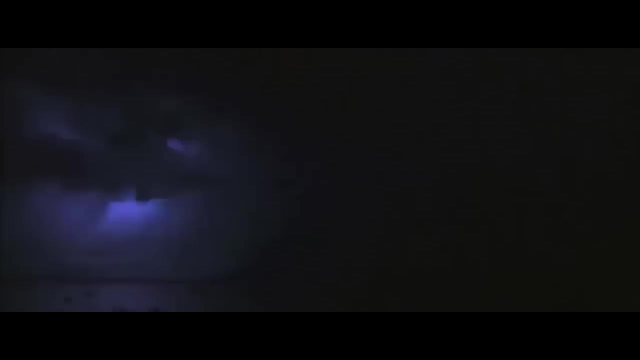 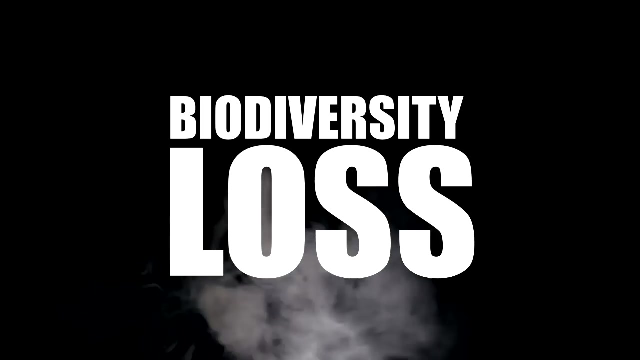 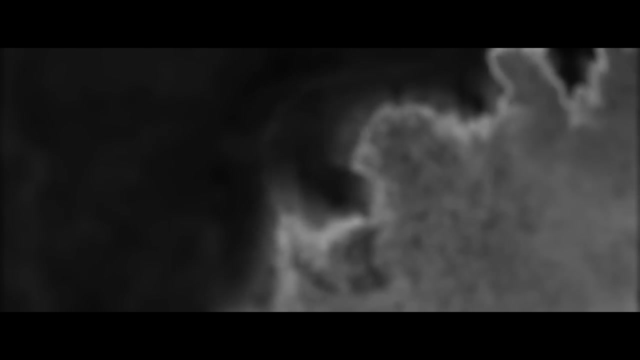 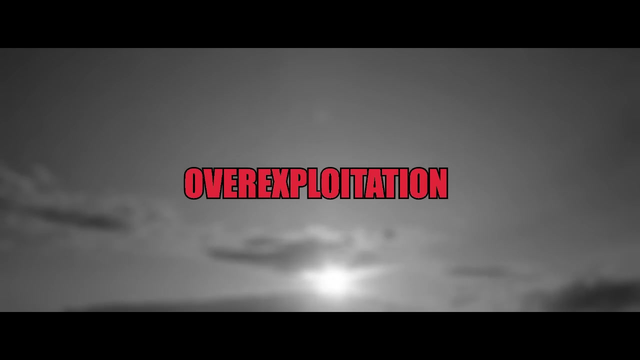 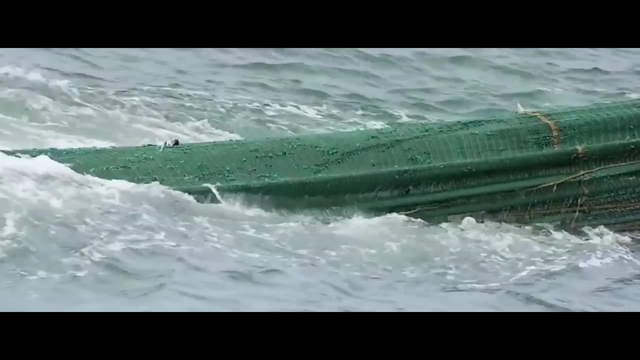 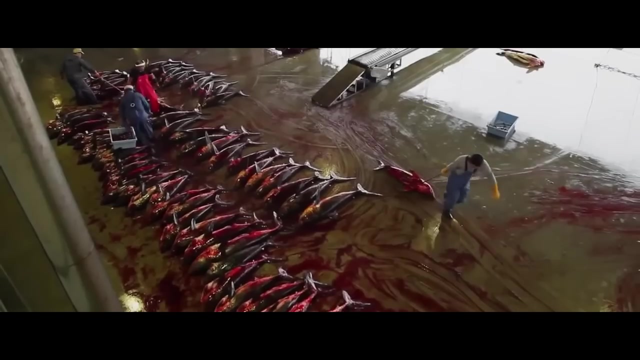 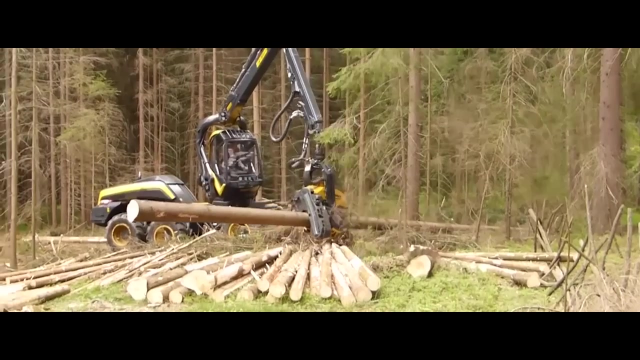 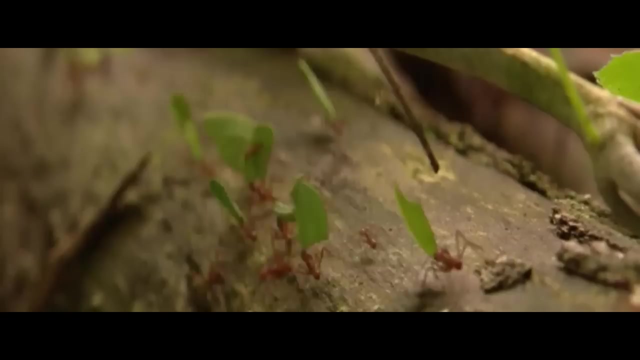 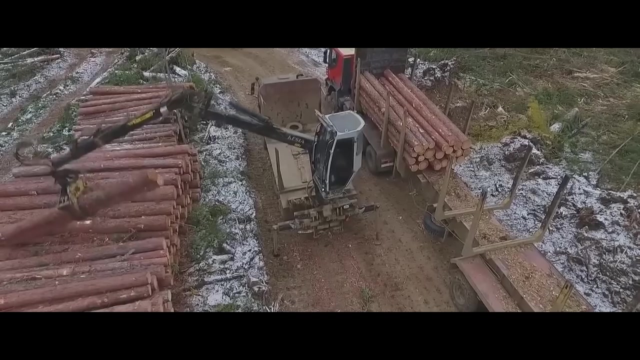 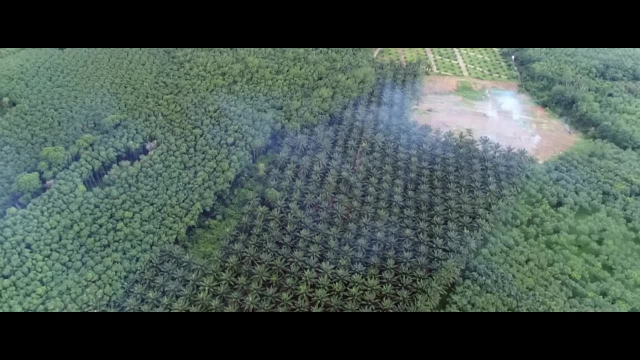 result of the natural or human activities such as earthquakes, land use, deforestation or agriculture. biodiversity is lost as a result of the natural or human activities such as earthquakes, land use, deforestation or agriculture. biodiversity is lost as the ecological system supporting biological survival is taken away. 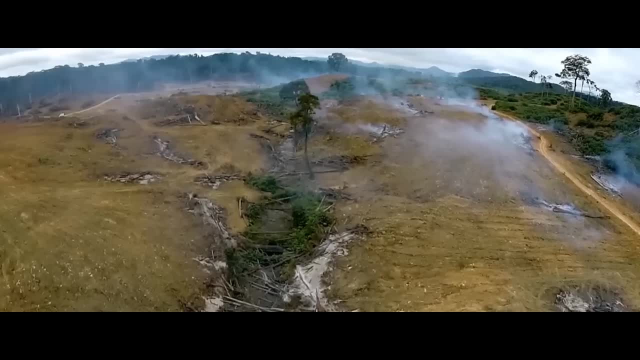 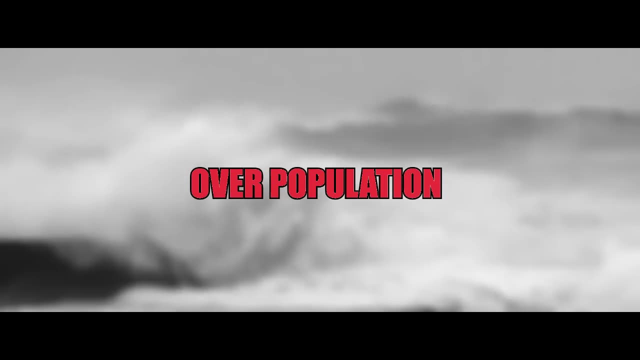 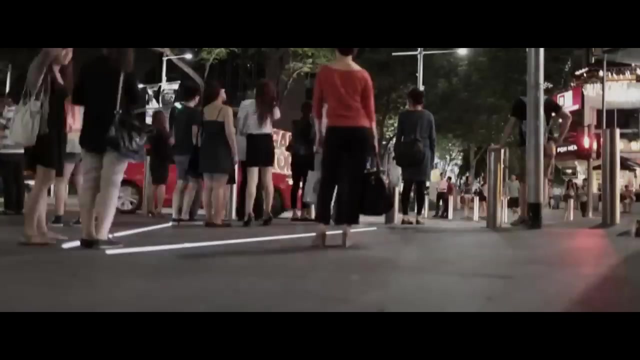 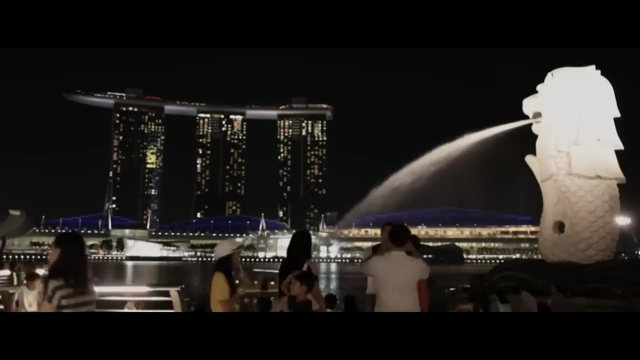 Even if only a small portion of an ecosystem is destroyed, the entire system's balance becomes vulnerable. Human overpopulation. Overpopulation has witnessed continued accro-outment into frontier forests, heightened pollution and destruction of natural ecosystems. That has considerably contributed to the loss of natural ecosystems. 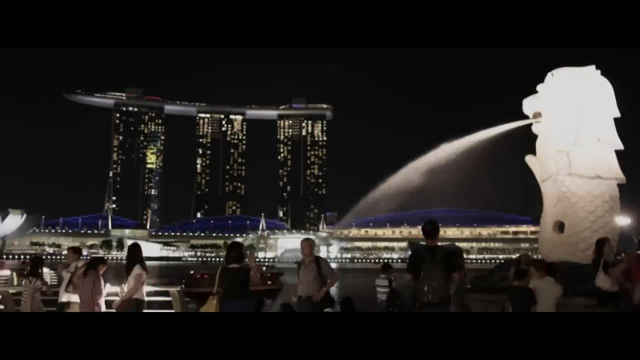 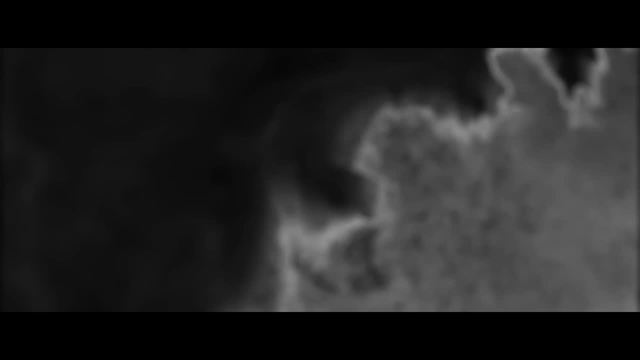 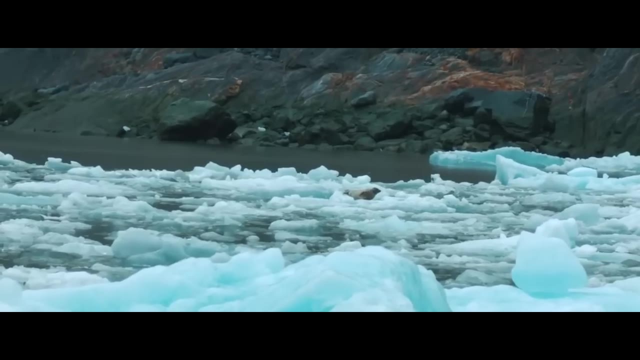 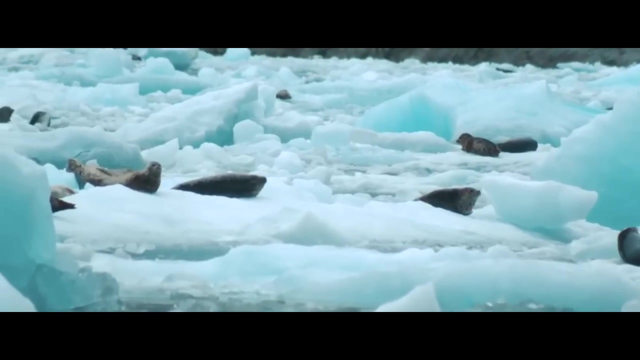 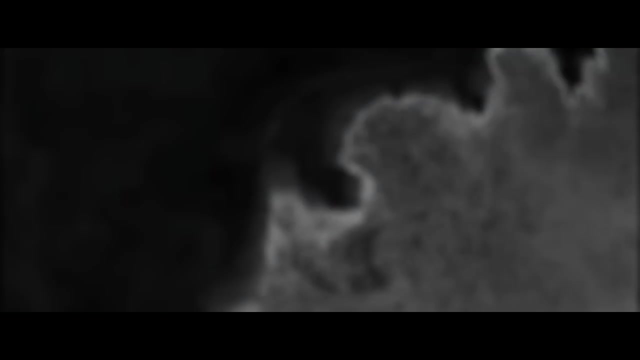 to the mass extinction of species. the number of threatened species persist to multiply worldwide, whereas some have completely gone extinct. climate change: when climate change occurs, temperatures can increase dramatically. when temperature rises, many different changes can occur on earth. it can result in more floods, droughts or intense rain, as well as more frequent and severe heat waves. 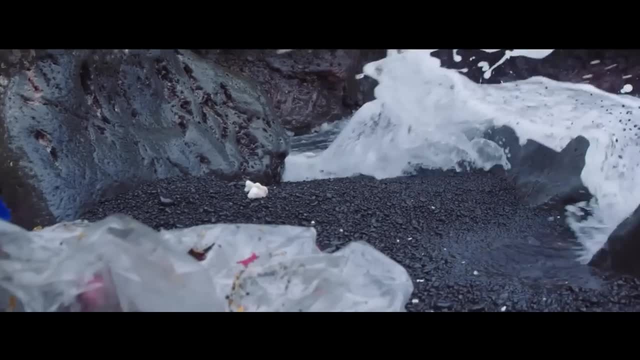 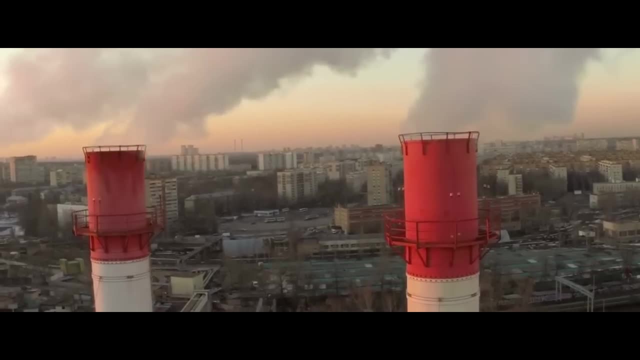 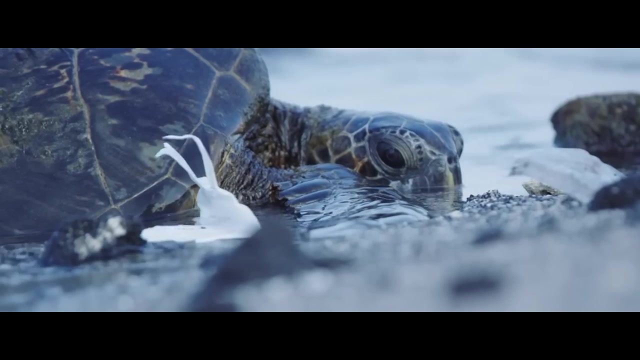 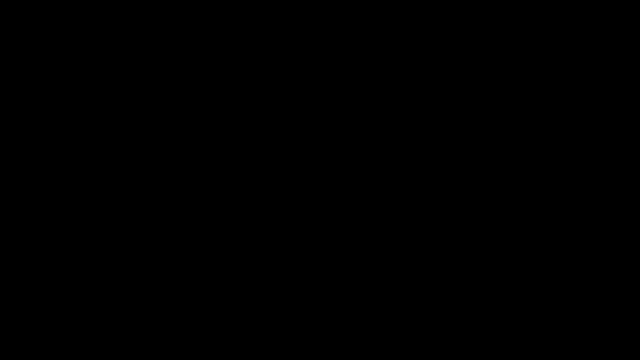 pollution. the various forms of pollution, including water pollution, soil pollution, air pollution, land pollution and agricultural pollution, simply destroy animal and plant habitats due to the toxic substances and chemicals released into the biological system, contributing to their eventual death. you out of these causes, one that contributes the most damage to biodiversity is 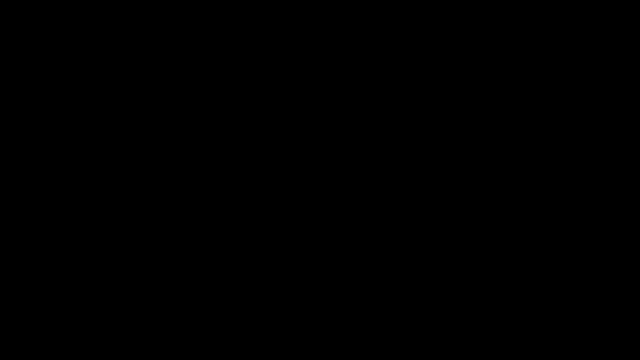 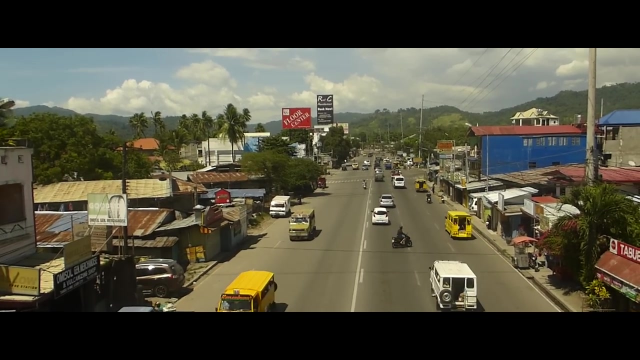 pollution, since it connects to the other major reasons of biodiversity depletion. we went to different places in our city to see if these activities that contribute to biodiversity loss are happening in our community. we also went to another park. we experiencing great Report on Lucia. we're going on our trek to Lucia. 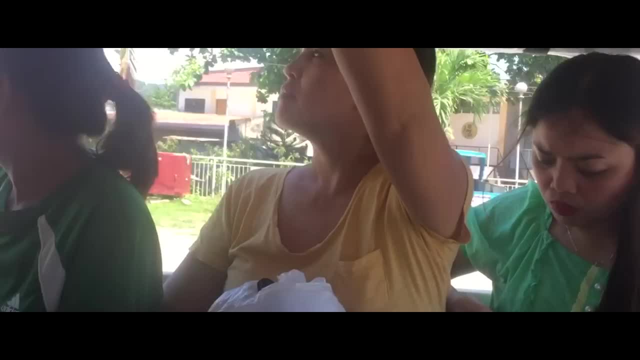 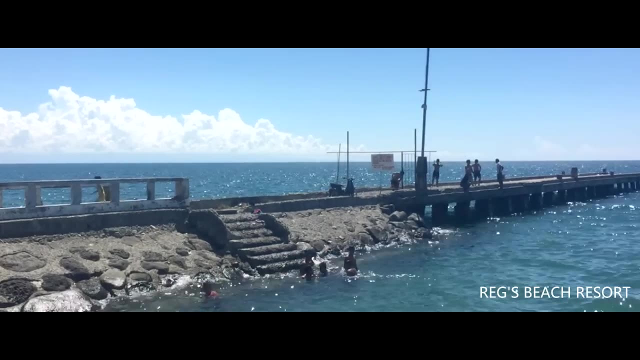 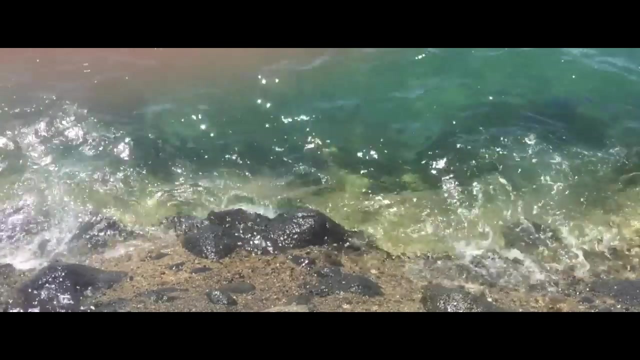 The winter before Christmas, when ohnectologies erupted, the forest started growing and the climate normalization of forests began. all this unknown. All bloggers are making a voice about the un öğrenden. We just showed our picture that we took last summer. Our value deepens now. 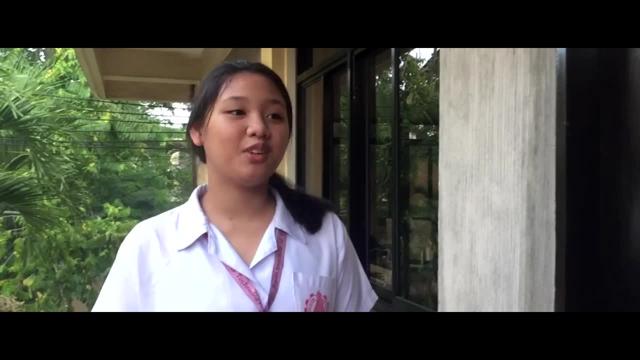 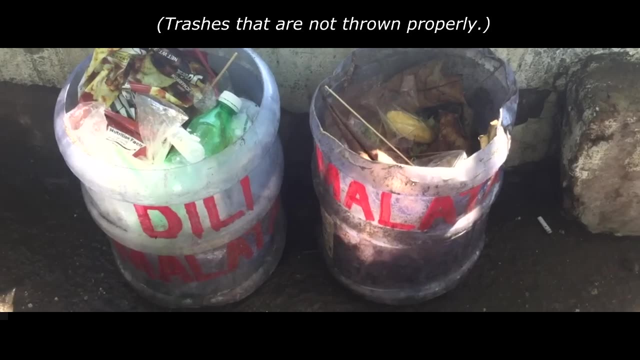 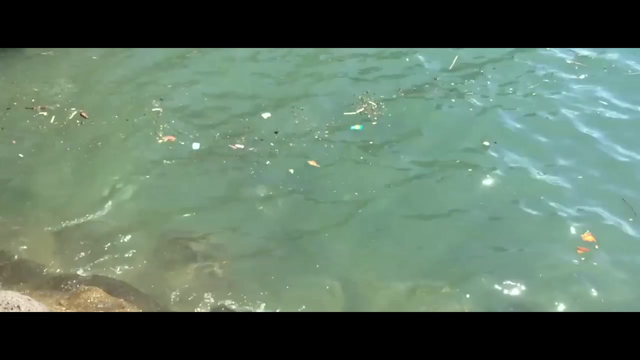 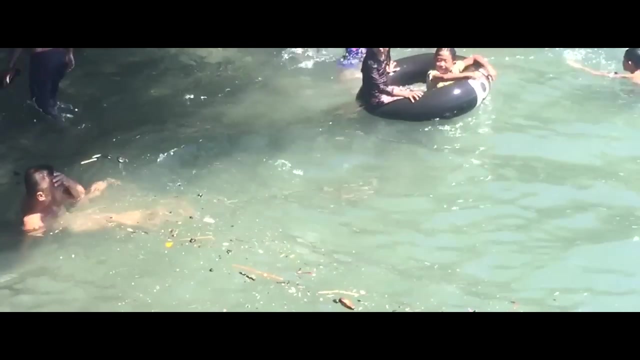 There are different places in Iligan, but this is the first time I've been to the Regs Beach Resort. There are a lot of happy people here, But in the end what we saw was trash. They were cooking and the kids were playing around. 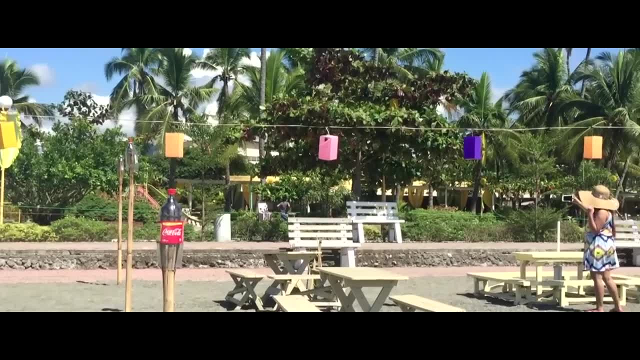 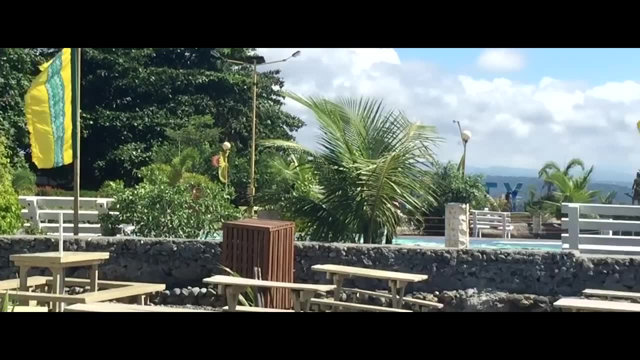 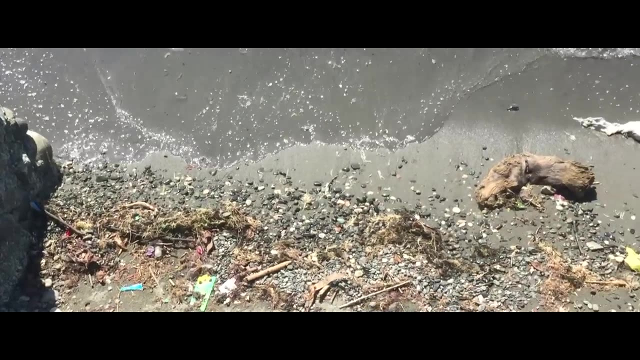 This is the first time I've been here. It's wonderful because there are many statues. There are horses, horses, jeeps. There are a lot of people here. I'm going to check out the beach And then I'm going to go to the sea. 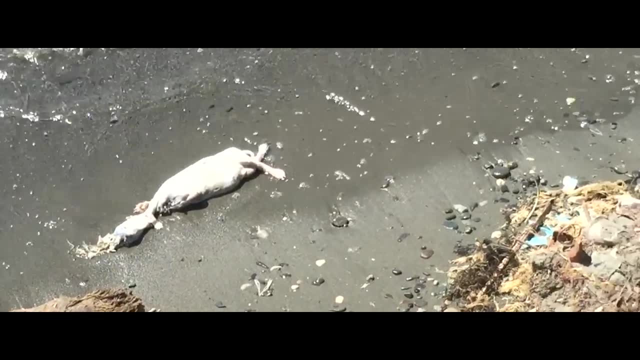 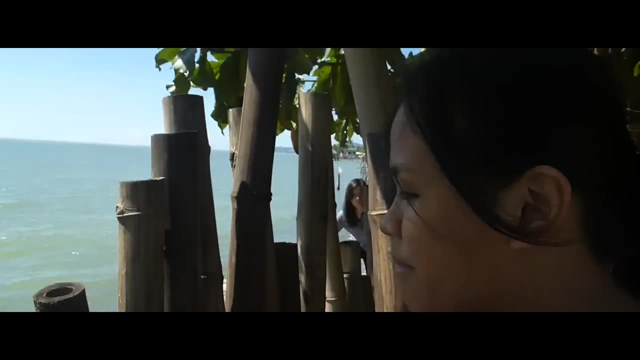 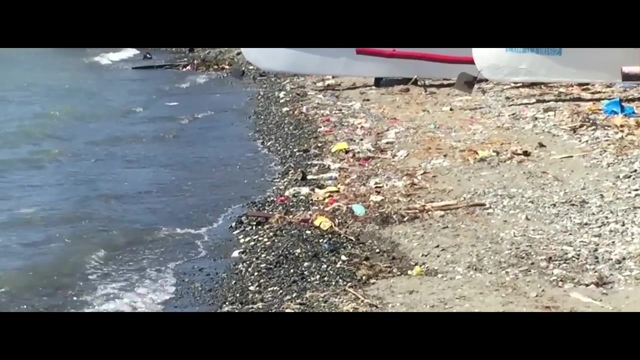 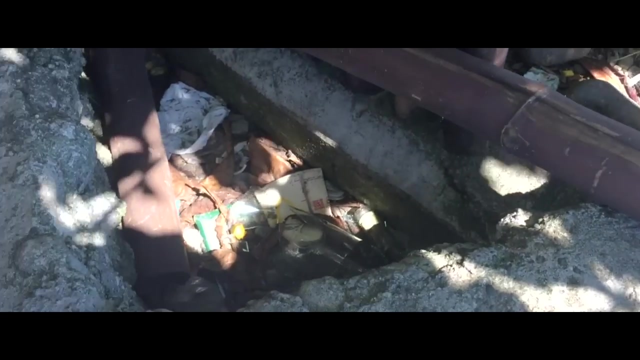 And then I'm going to look for the trash Guys. we're at the Biodiversity Lost Day Where Biodiversity Lost Day. There's a lot of trash around here. The tributaries are everywhere. There are a lot of people. 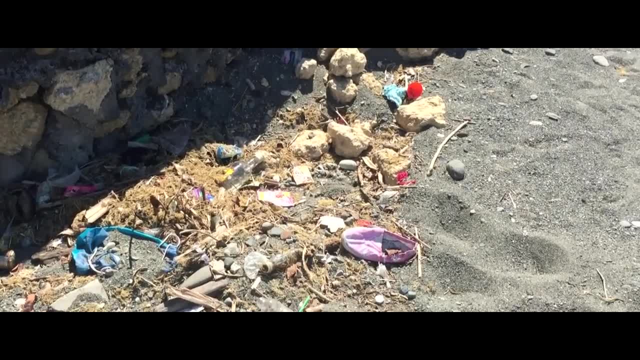 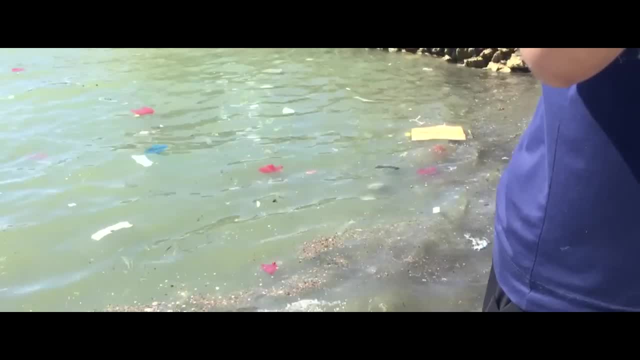 I'll just go and check out the beach. It's very crowded and it's raining. I think it will rain sometime. There's another beach. Look at that. There's a beach here. It's very crowded. Look at that. 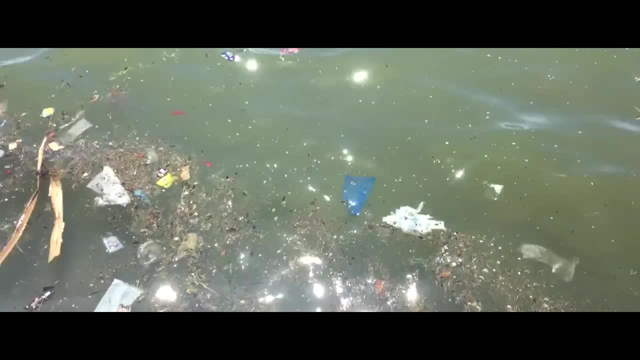 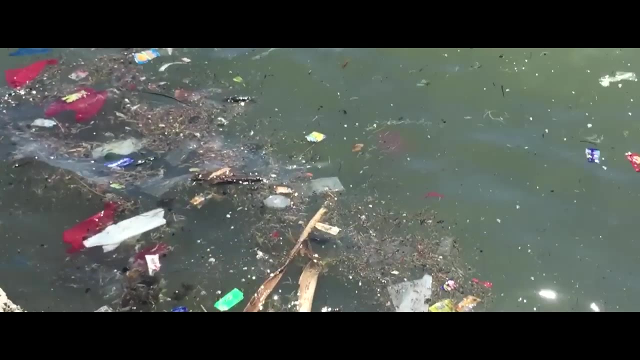 It's very crowded. It's raining. It could rain, But it's very sunny, It's raining. Oh look, someone is walking around. Oh, it's so beautiful, It's beautiful. Oh my goodness, It's like we're in Palau. 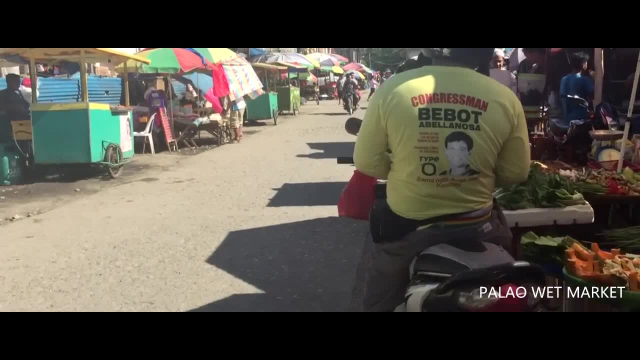 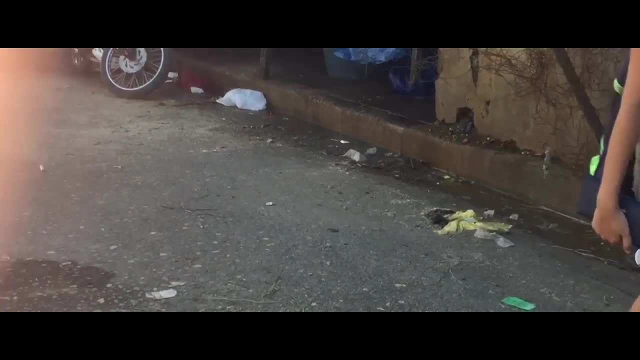 We're in Palau Market in Bagsakan, Dapit. Here it's so beautiful, There's a lot of flowers. When we go to Bagsakan, there's vegetables and fruits. Guys, look over there, The sides of the market are full of trash. 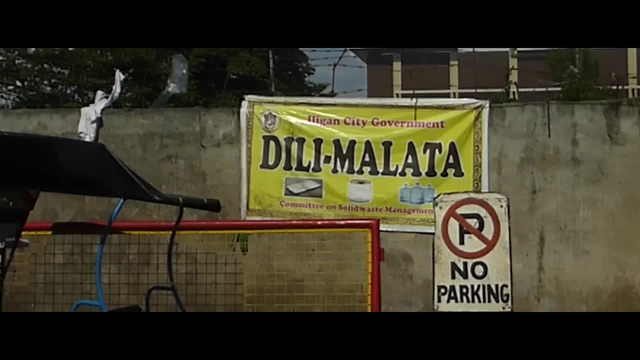 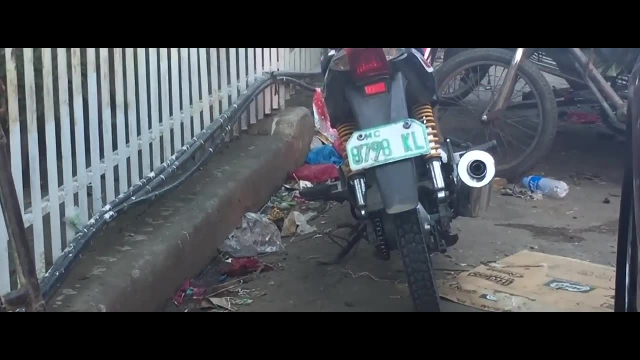 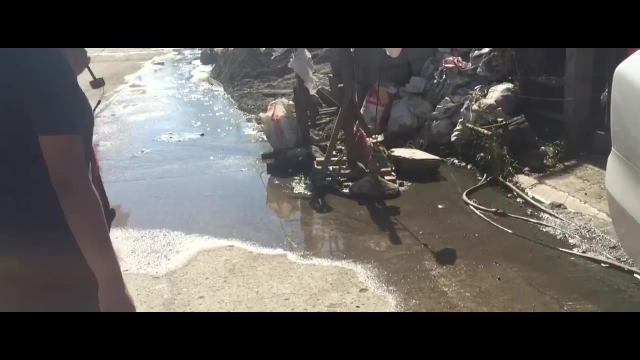 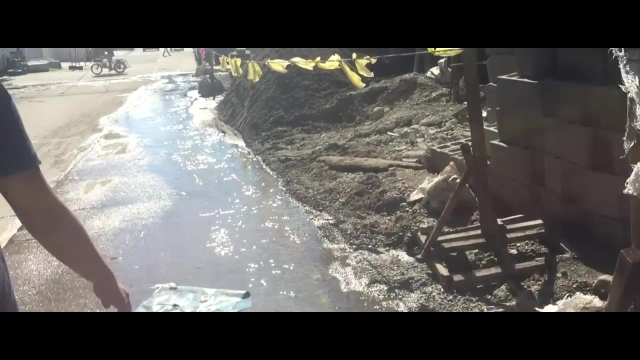 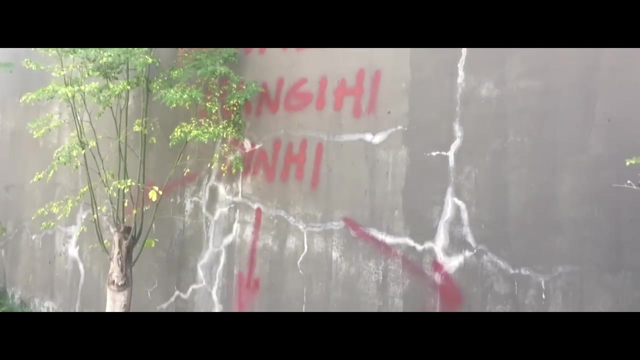 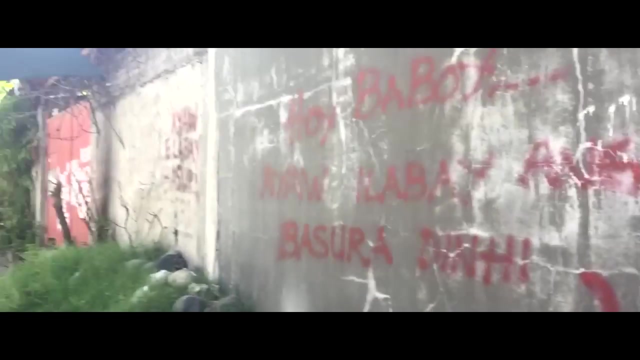 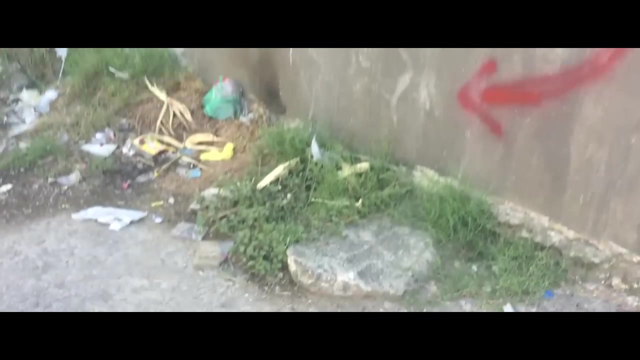 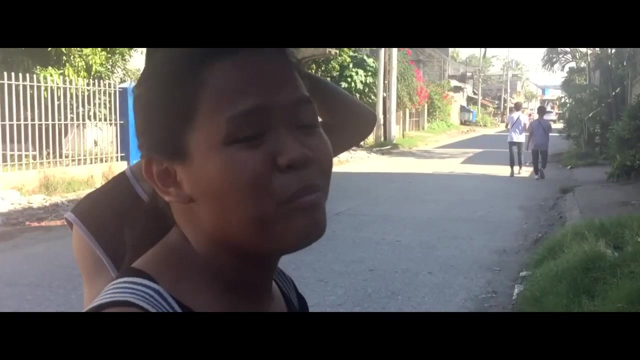 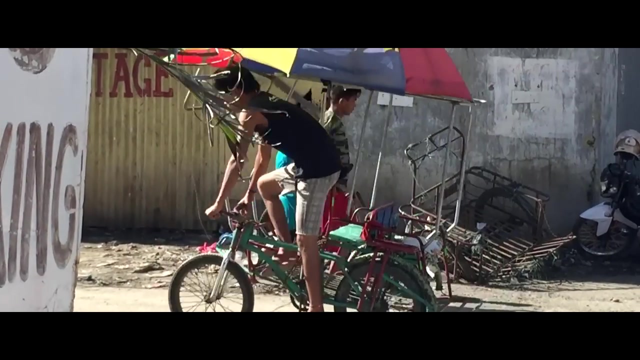 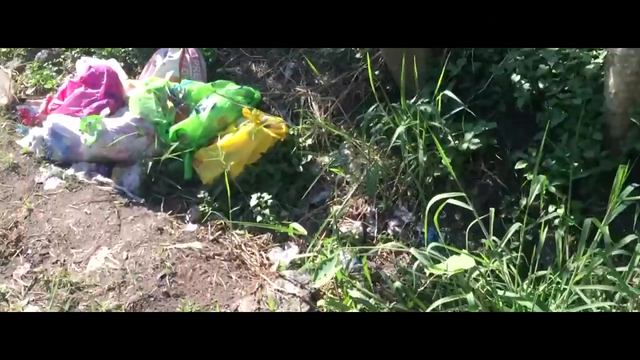 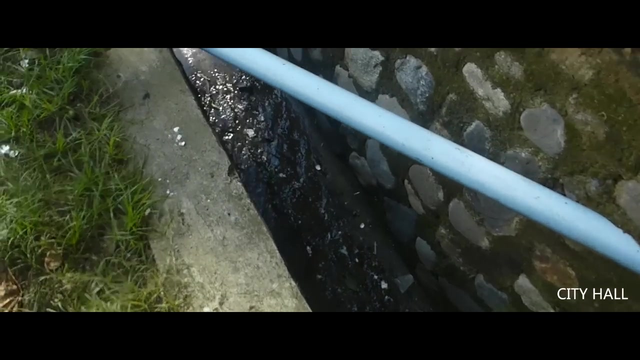 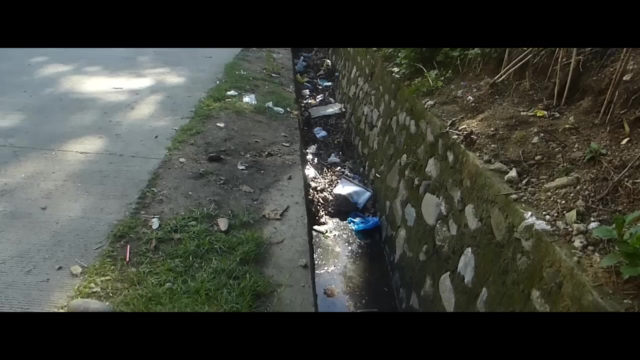 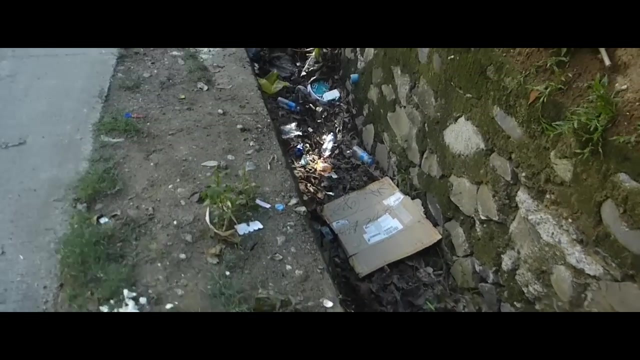 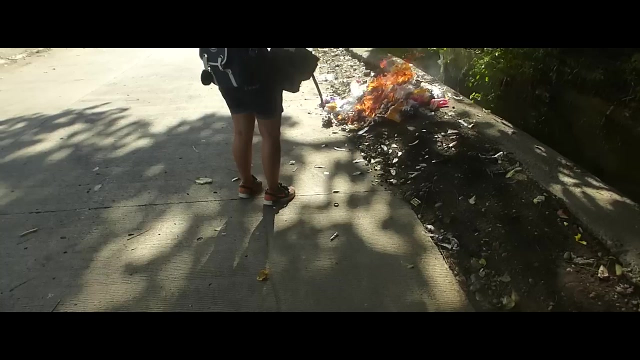 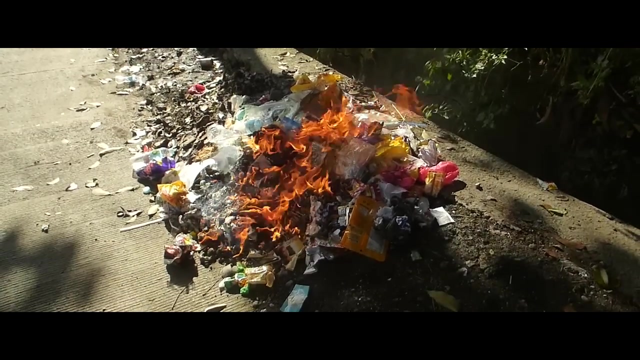 Yes, Save water. Hey, Oh, my god, a girl. Oh, You thought no limp you can turn on, but no, It's dirty y'all. well, hey, hey, it's real. Hey, Do they have some money? Guys Burning of plastic, my god, my god, guys, this is seriously. 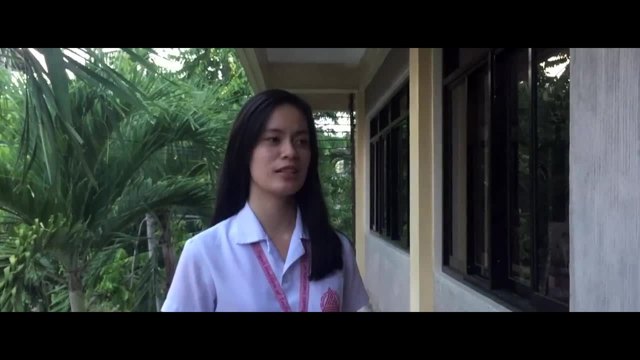 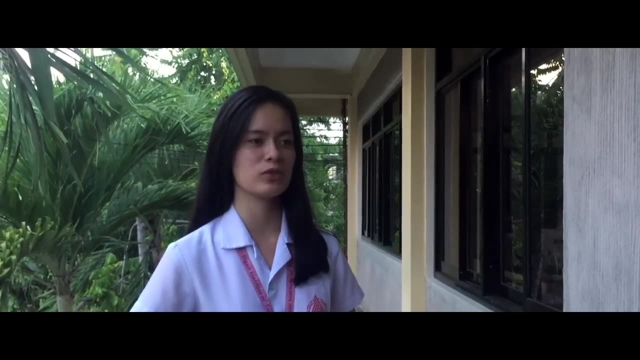 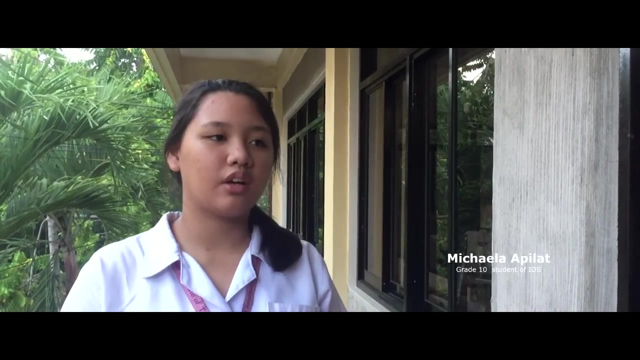 So the number one Say vegan, a small parts of the silly gun, but It's a gossip dude, magic crushes everywhere, So probably you can issue some city, most especially some bigger city spa. we have seen many when I'm wearing. Evidence has. no, I don't want you to tell you what I discipline. 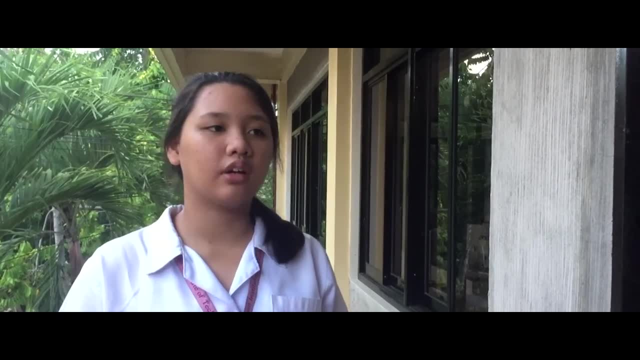 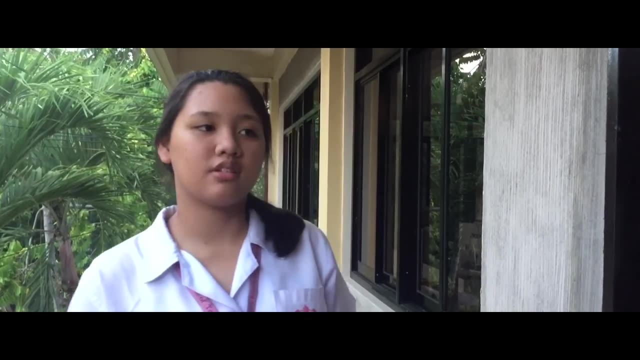 Then, first of all, good for my great talk, and I'm my own- a community, Clean and green. it's not a brief down there. Okay, the, but we should start with ourselves. What do you need? Shia station, you know. so I don't want to. 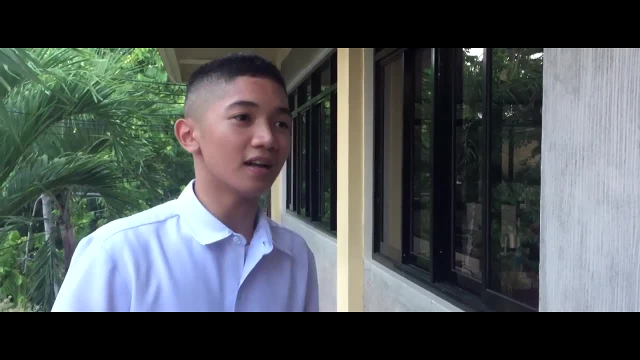 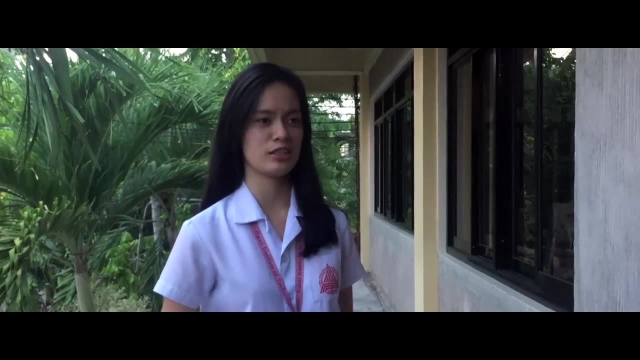 Can I be talking about? not so? so I don't understand. not to be fixed, Okay, but I think when it's just a tongue, younger generations as humans, I don't get much start on change. Even the school, the bomb will get out of the trashes everywhere. I'm asking: sign up. 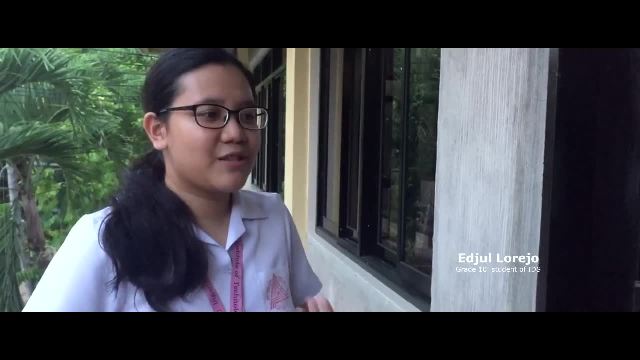 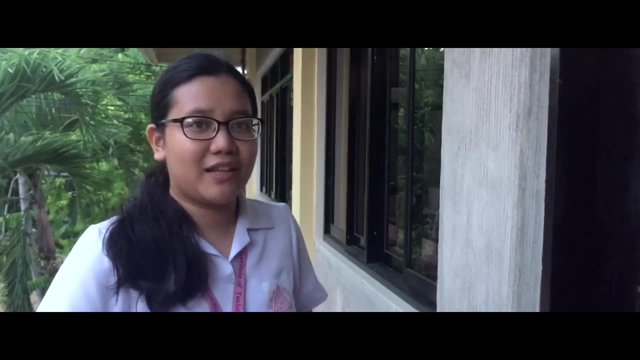 I'm sorry but I don't want to kill it. some of them as soon as the pancetta. I'm gonna take action because the cabal Utah. we are educated. so Even if you think that Canada moves more things taking squatting, why change no? 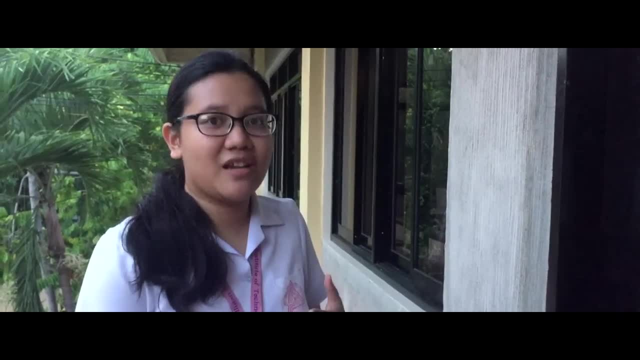 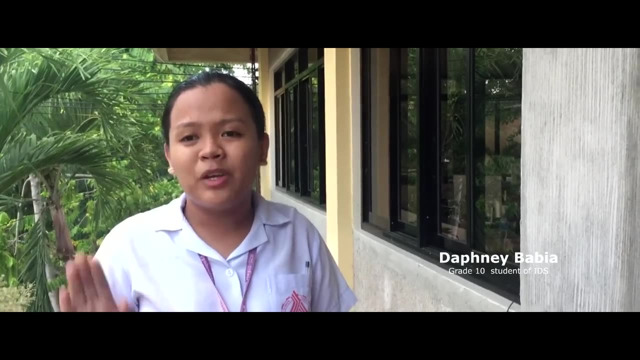 Imagine she change. we are gradually Making a change or an impact on mother earth. some of the town has a gilk on Allah by basara. Danny Caballon say: biodegradable and biodegradable. Sukarno 있는 sana Shutty, it's not gonna give a momet. 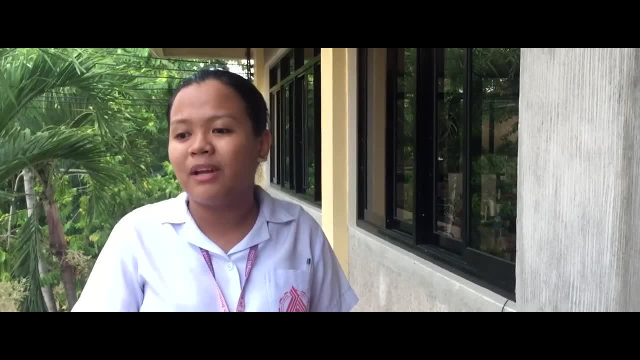 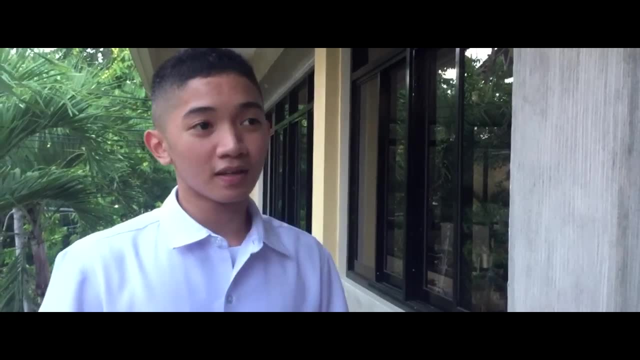 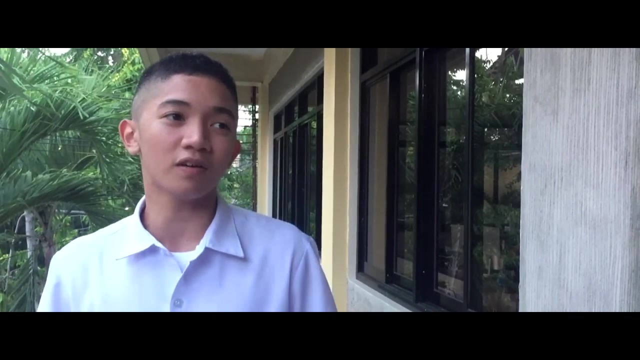 You know I'm on the other earth. What the mocha dialogue? up and get a gap and a gap in my distance on a calip pounding hugo Kyle. As as as mga people, If we are still young, we should take care of ourselves, because it would be a waste not to take care of ourselves if we don't take care of ourselves. 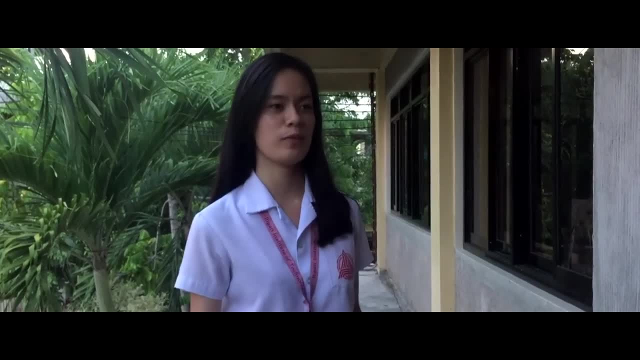 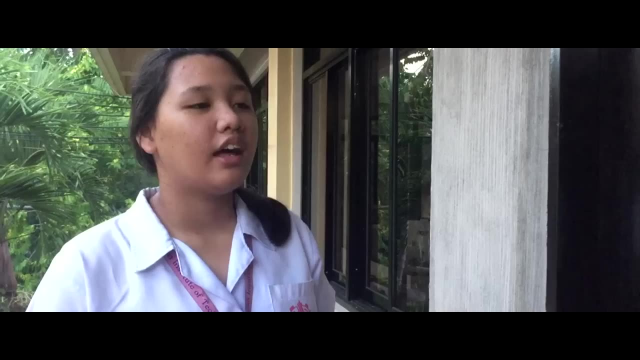 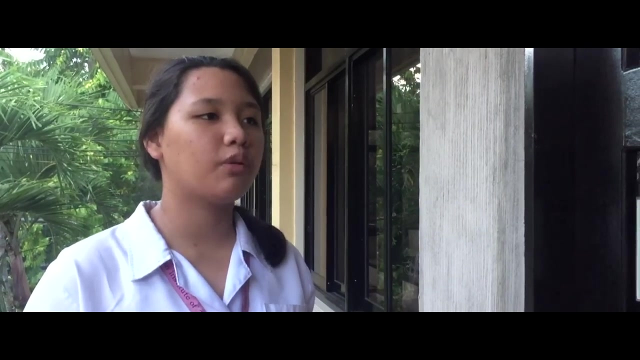 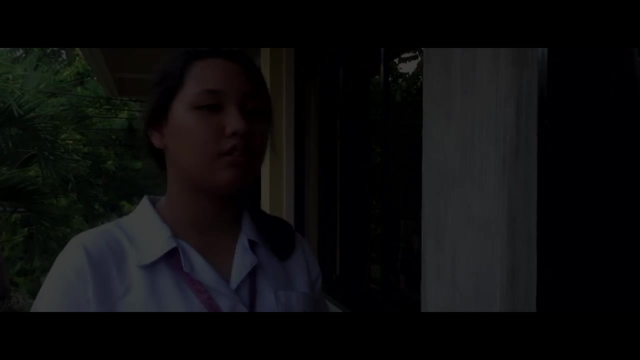 We should also take care of our environmental issues, because it is our responsibility as humans. We are assigned by God to take care of this earth, And I hope that this message reaches to all the people who watch this. I hope that they would be concerned to our environment, be concerned to the people who live in that environment. 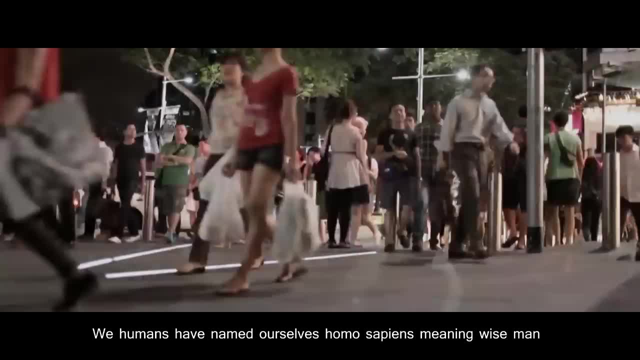 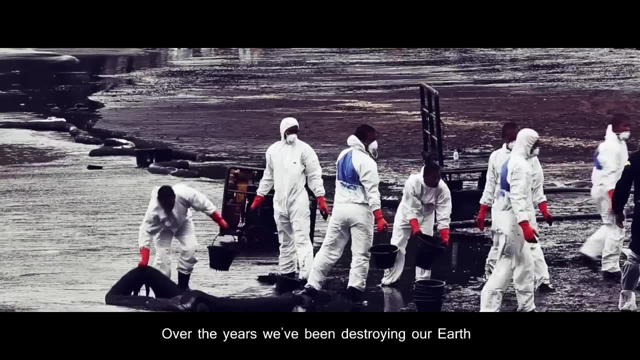 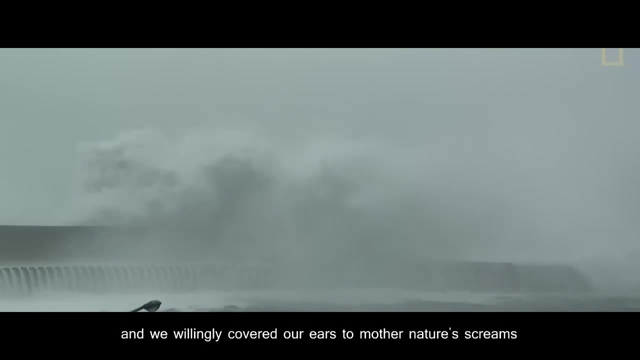 We humans have named ourselves homo sapiens, meaning wise men. But is man really so wise? Over the years, we've been destroying our earth Day by day. animals go extinct, Resources are being damaged And we willingly covered our ears to Mother Nature's creams and closed our eyes to all of her health-wanted signs. 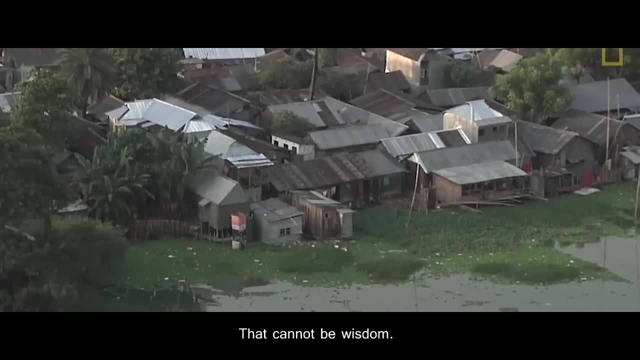 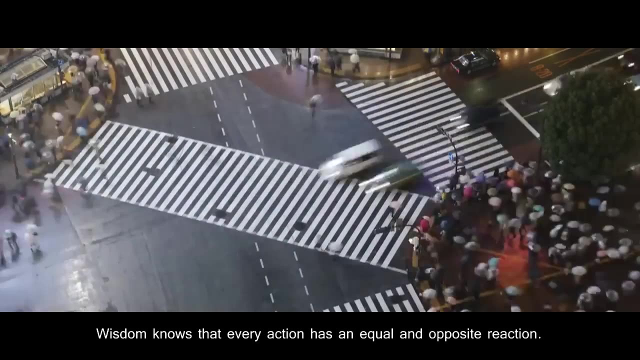 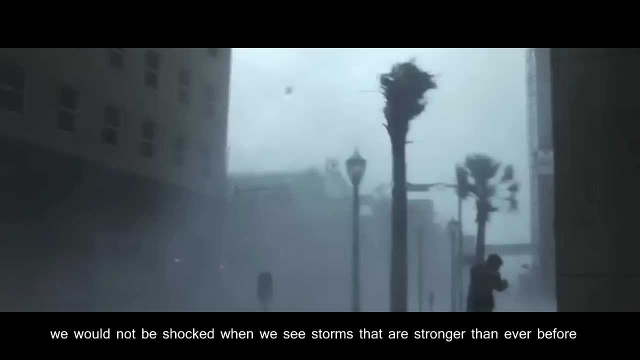 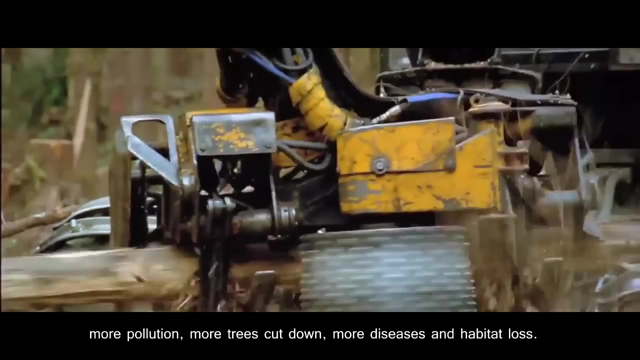 That cannot be wisdom. Wisdom knows that every action has an equal and opposite reaction. So if we were wise, we would not be shocked if we see storms that are stronger than ever before, Or more droughts, hurricanes and wildfires, more pollution, more trees cut down, more diseases and habitat loss.